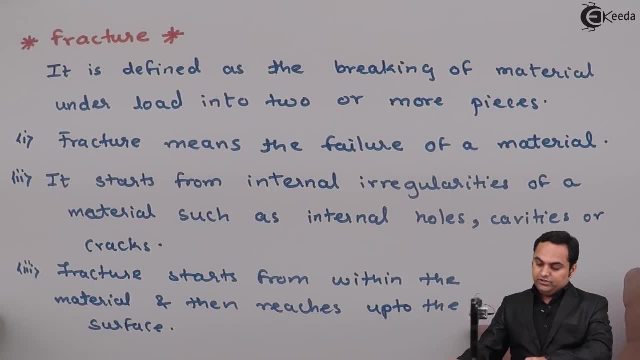 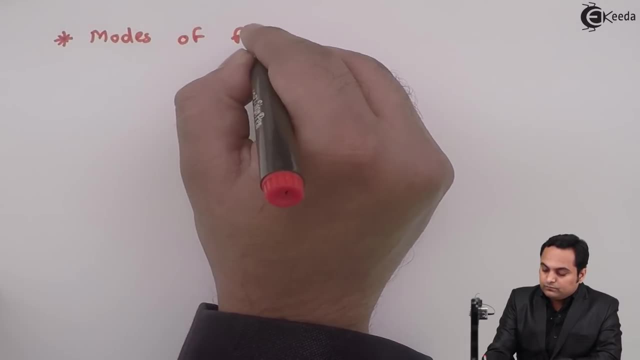 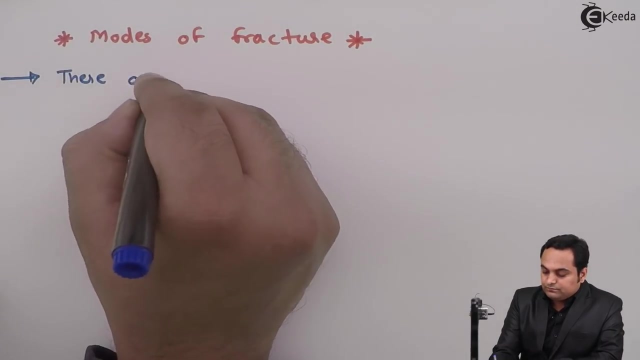 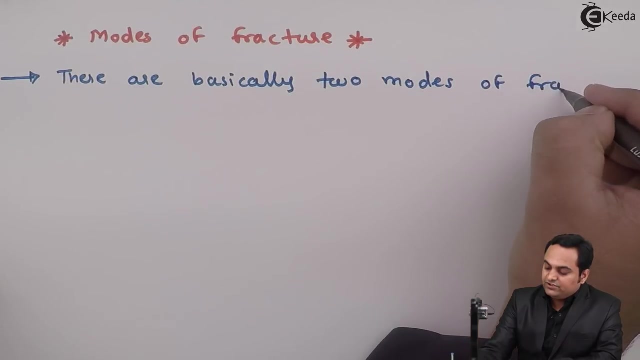 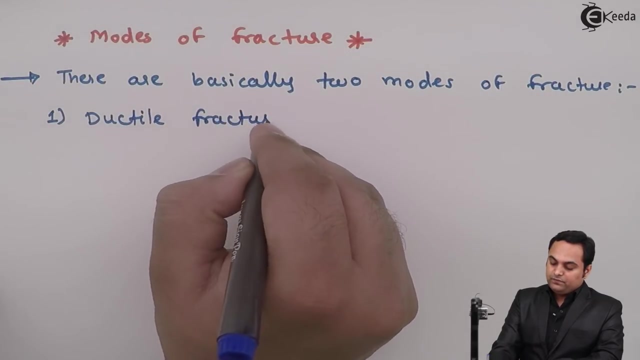 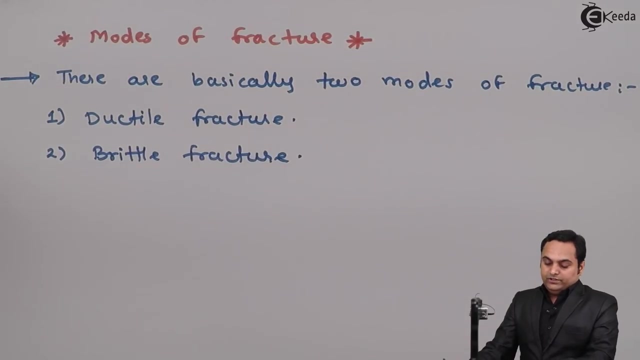 Now, once we have understood the definition, now I can start with the modes of fracture. In the modes of fracture I will write down: there are basically two modes of fracture and they are ductile fracture and second, brittle fracture. Now to understand these modes in detail, here I will write down: 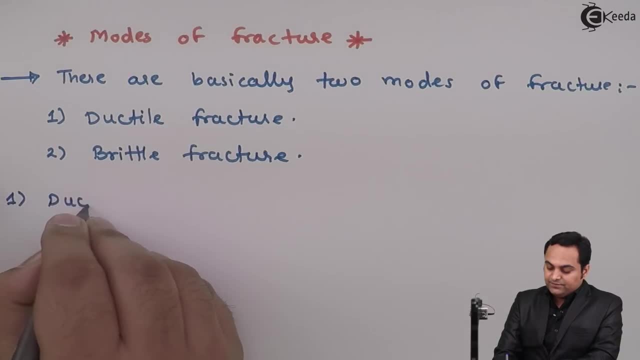 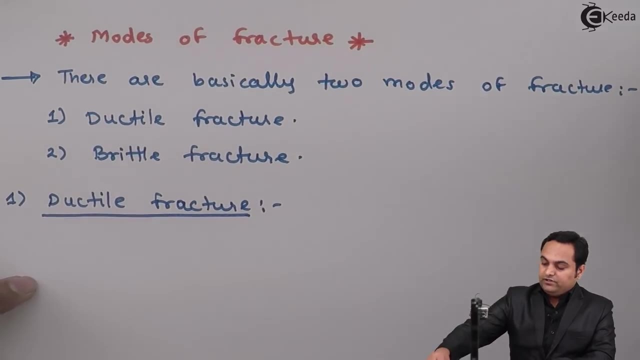 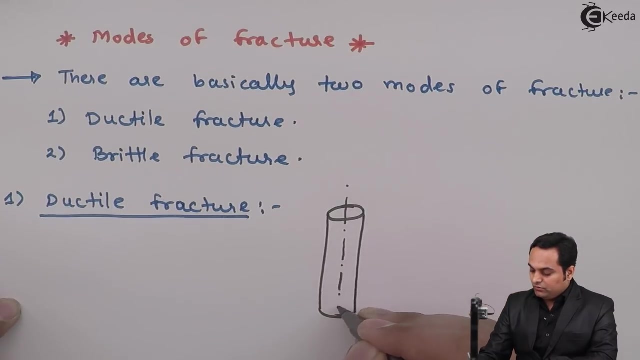 The first one is ductile fracture, one that is ductile fracture. now for ductile fracture here, if we consider an element, or I can say a rod, which is stress, here we have a rod. this is the axis of the rod. now, if we apply tensile, load over this rod. if we are trying to pull the road by applying tensile, 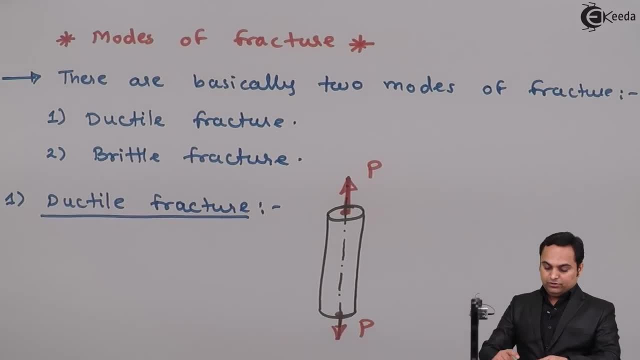 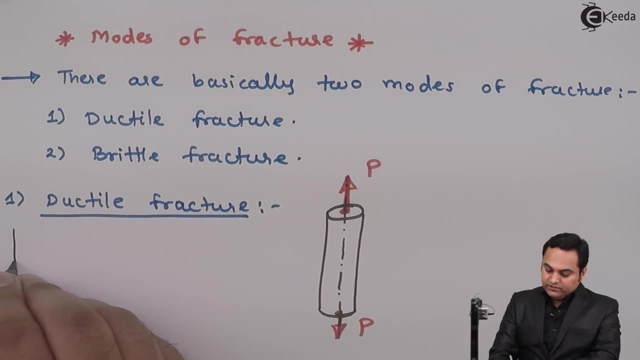 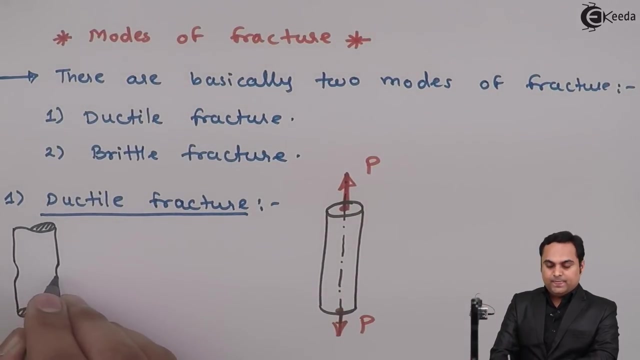 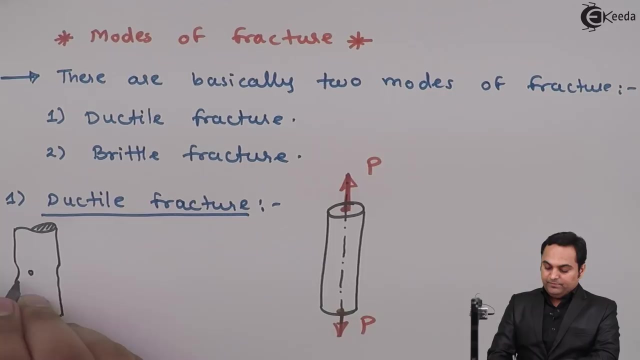 load. then what will happen is- I'll draw the different modes. first of all, the diameter. it will slightly decrease under theoured of the load. the diameter will start decreasing. if there are internal holes present, then the crack will go on forming and this diameter will be further reduced when the load value increases. so 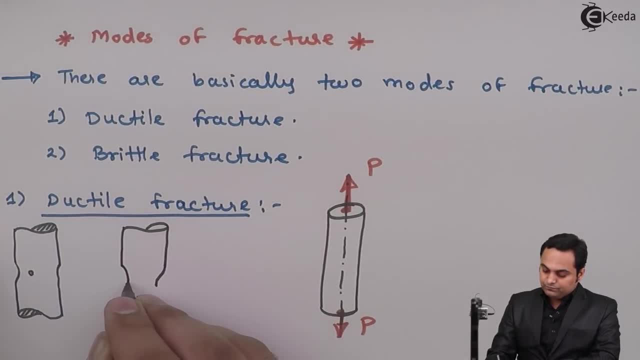 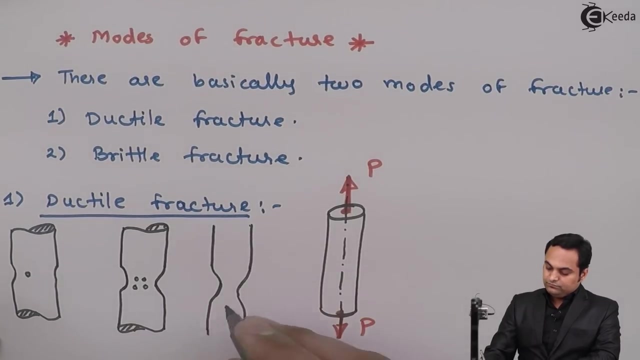 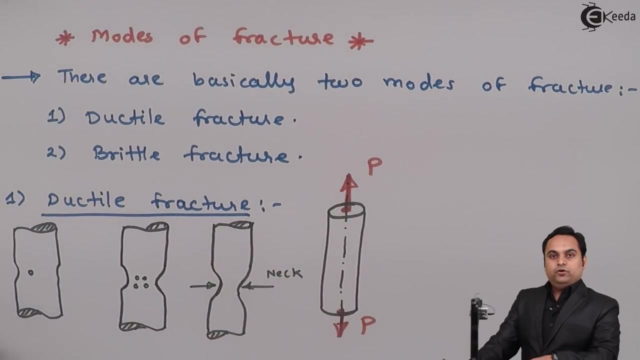 in the next stage, more number of holes will appear inside the material. or, if there are more number of holes, there would be cracks develop. next, finally, the diameter will be reduced to a very small value. you have this region- it is called as the neck- which is formed. that is the 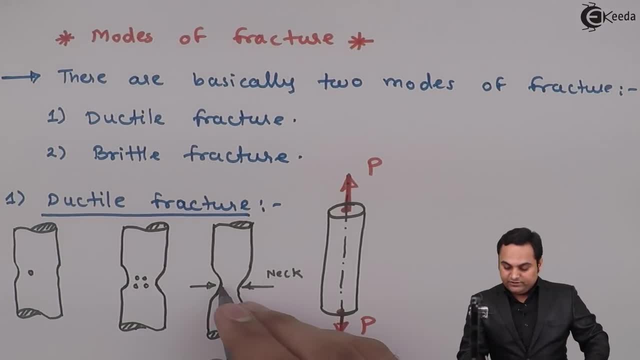 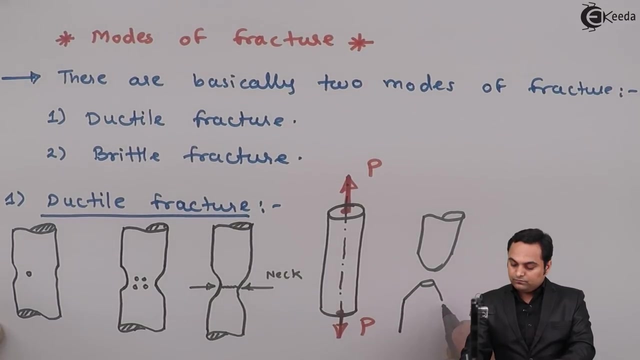 diameter has reduced to a minimum value and after this stage the cracks would be formed. and finally, when we increase the load value, then the material will break. and the material will break into this form and here this arrangement, this is called as cup, and here we have cone arrangement. that is, once we have applied. 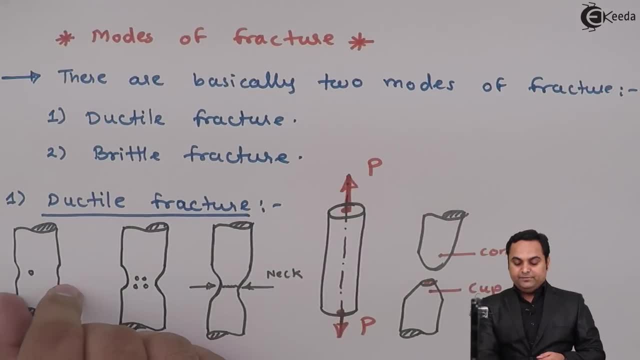 the load, the length will go on increasing, diameter will go on decreasing and then if there is internal holes, because of that the stress will go on increasing. again when the load is applied or load is increased, the diameter will go on decreasing. finally, there will be a neck form. that is a very small diameter and again, if we are applying the load, 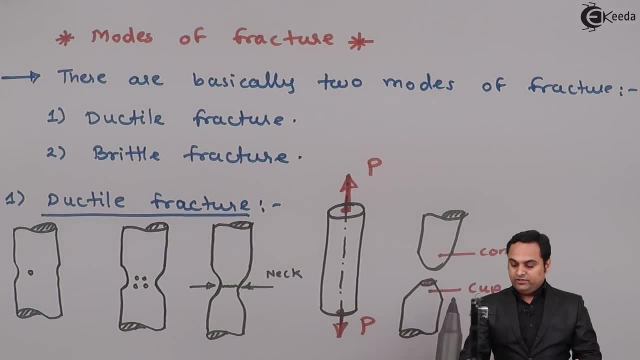 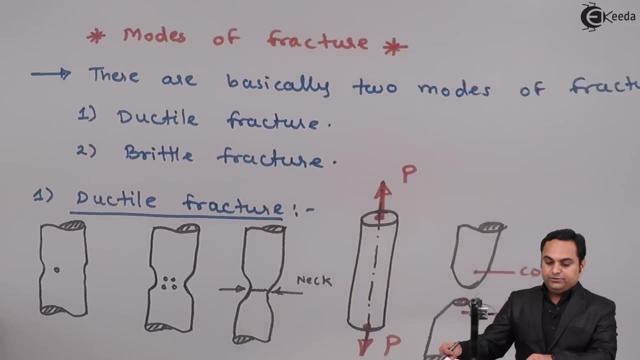 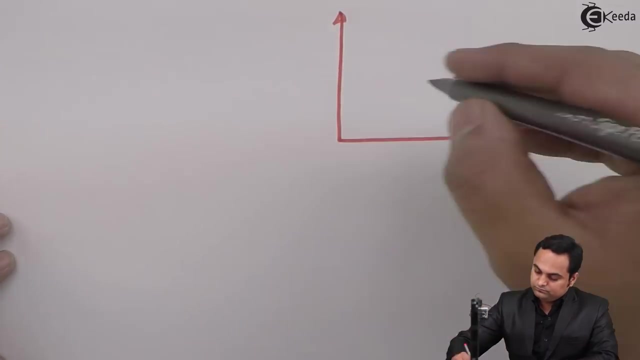 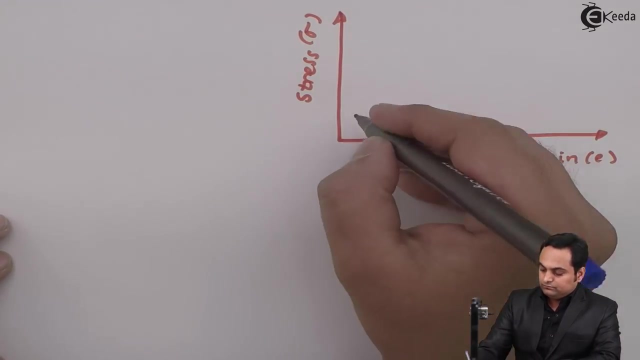 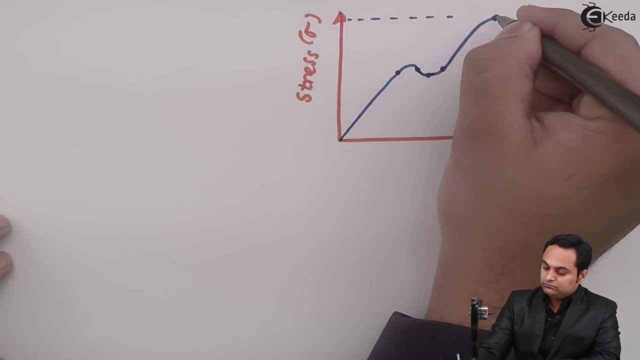 then the material will break into two halves and here we have cup and cone arrangement. so this was regarding the ductile fracture. next I can draw a graph related to this: uddress vs strain graph. now here we have point O to A, then B, C, D, E and F, where F is called as the 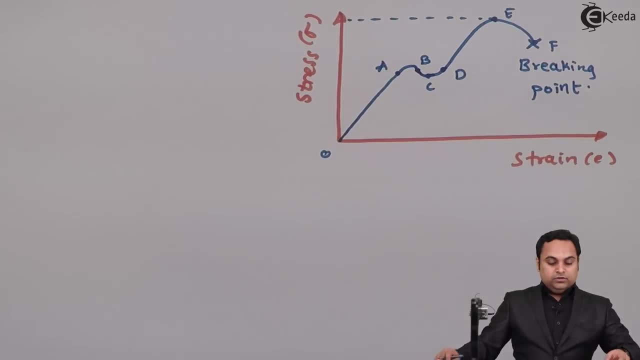 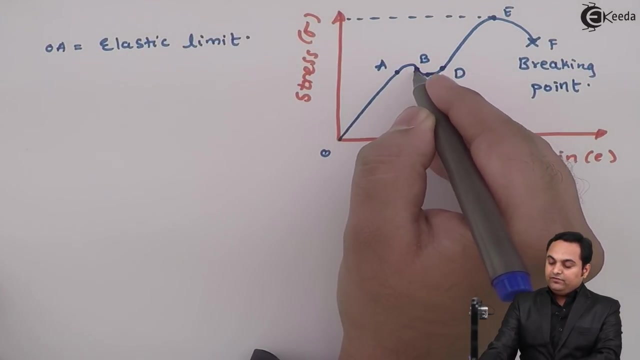 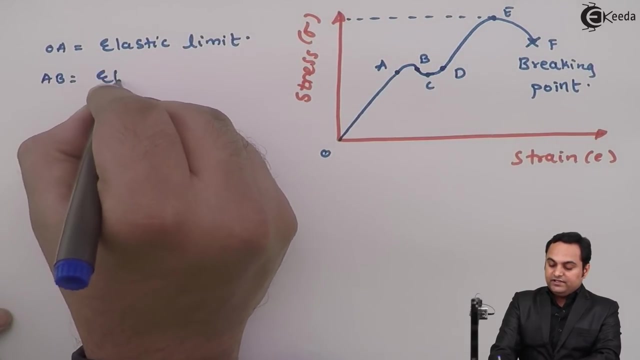 breaking point. now, once we are increasing the stress value, strain increases. 0 to a is called as elastic limit, next a to b. here we have another region in which, if we are applying the load and then when the load is removed, material will go back to its original shape. so here, after this, we have a to b. again. this is an elastic region. 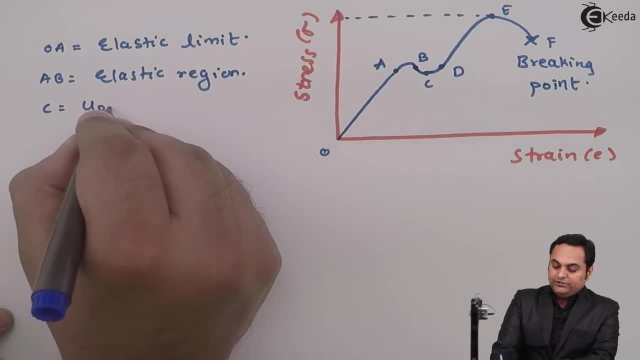 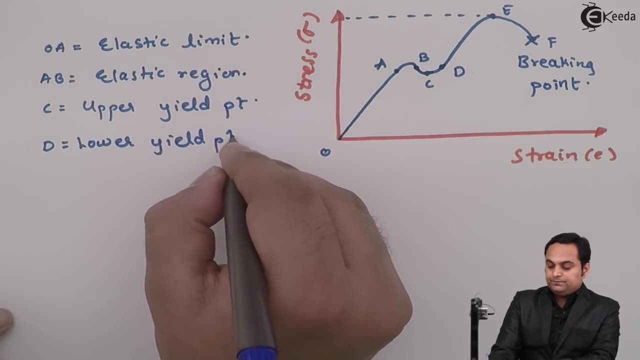 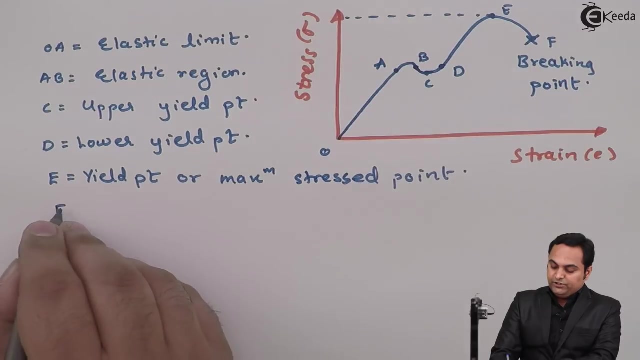 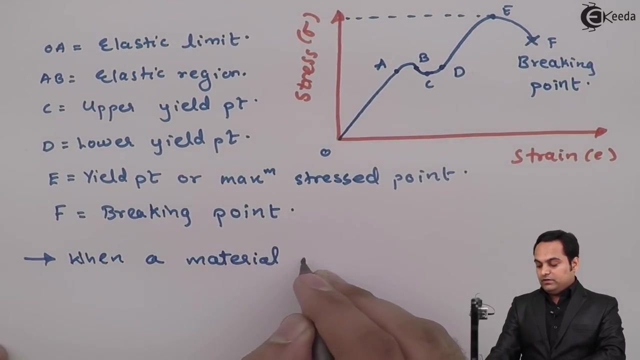 next c is called as upper yield point and d is called as lower yield point. then point e, it is called as the yield point or maximum stress point, and finally point f, it is called as the breaking point, where the material will break into two parts. so when a material, when a material is subjected to ductile fracture, it will follow. 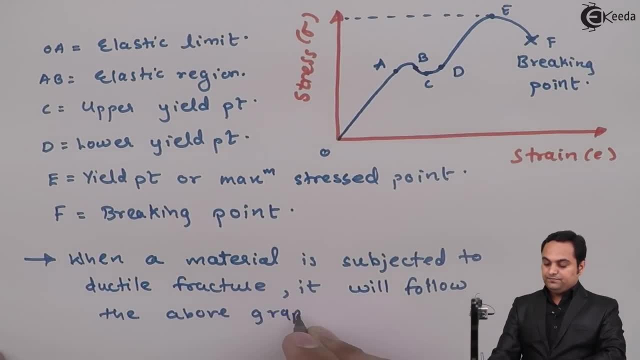 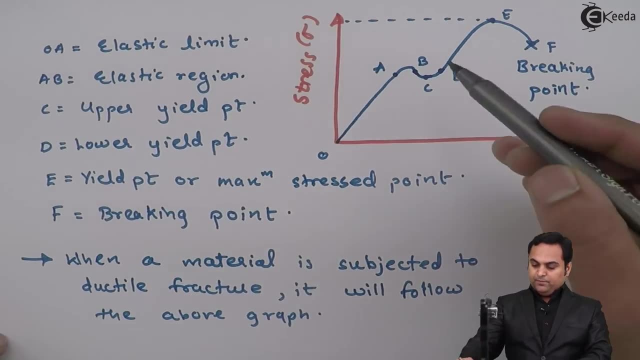 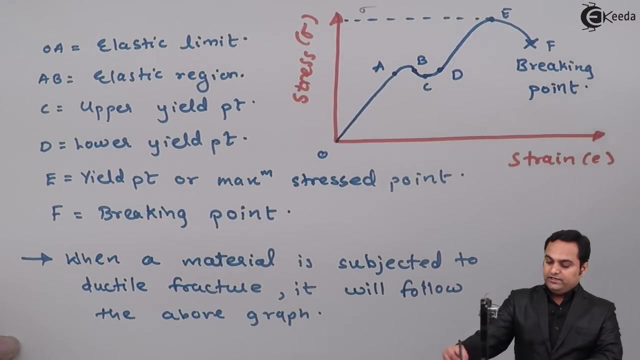 the above graph which I have drawn here. so now, here we have seen that when a material is subjected to ductile fracture, it will follow the above graph, that is, the material will follow this nature where we are getting at point e, the stress value as maximum, and if 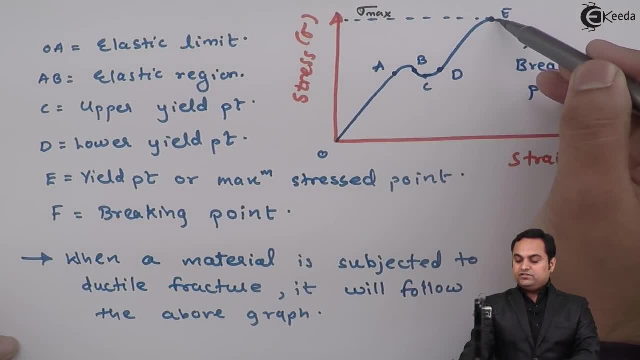 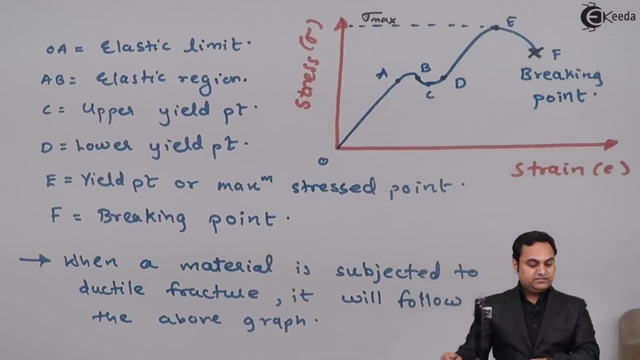 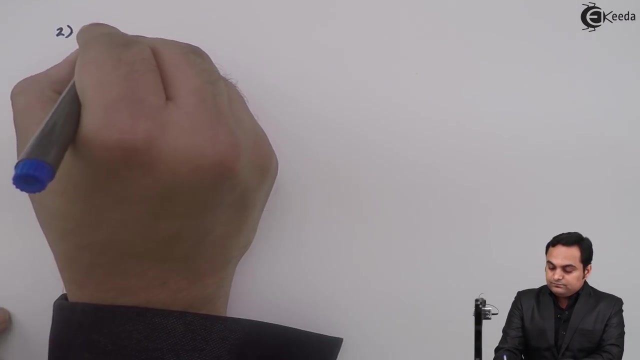 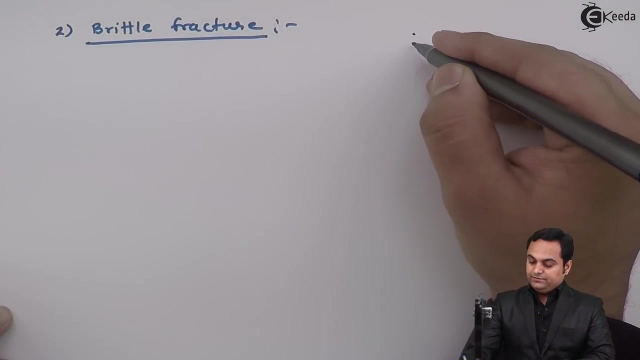 the material reaches maximum stress value, then, even if the stress decreases, there is a point at which the material will finally break, called as the breaking point. so this was for ductile material. now let us see the brittle fracture. you now for brittle fracture. let us consider a material which is brittle. 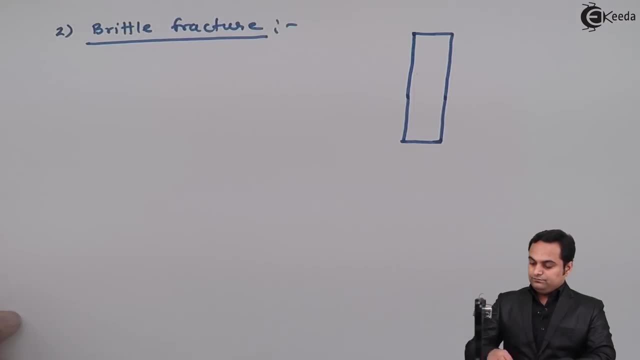 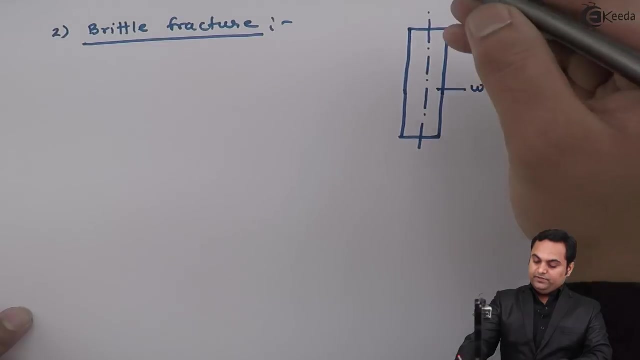 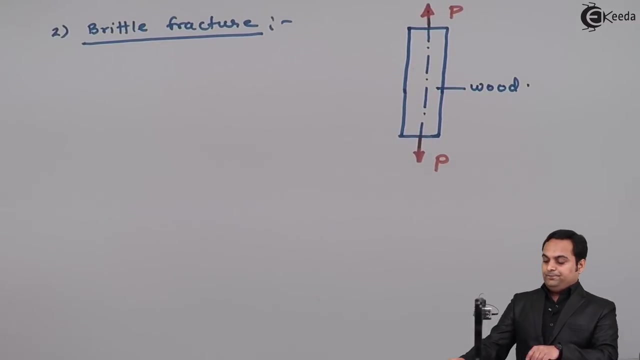 this is the axis of that brittle material. now, let this material be wood, because we know that wood is a brittle material, and let this word be subjected to short load, as shown in figure. this is a tensile load. now, what will happen is when wood is subjected to tensile load. first of all, it won't show any physical 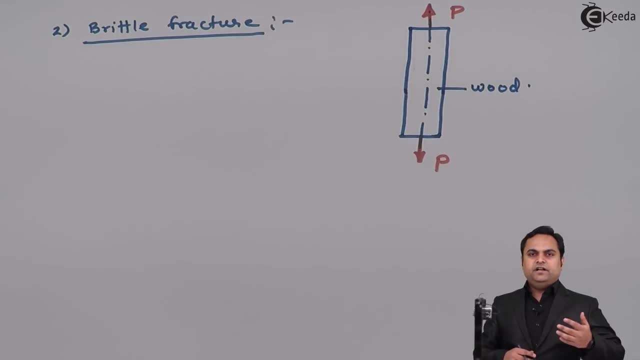 deformation. that is the property of brittle materials that at first, when the load is applied and the load is going on increasing, the material will not show any physical change. but suddenly, after some time, what may happen is, when the load increases, the material will break suddenly and that will result in its 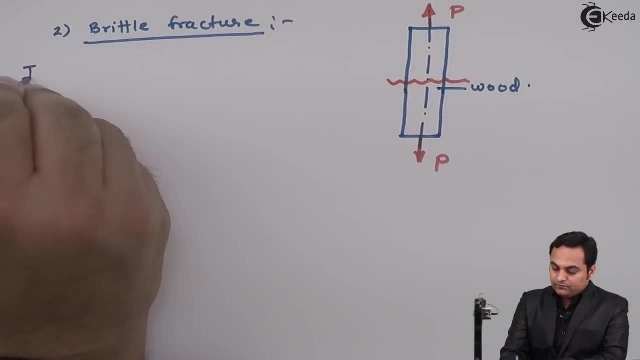 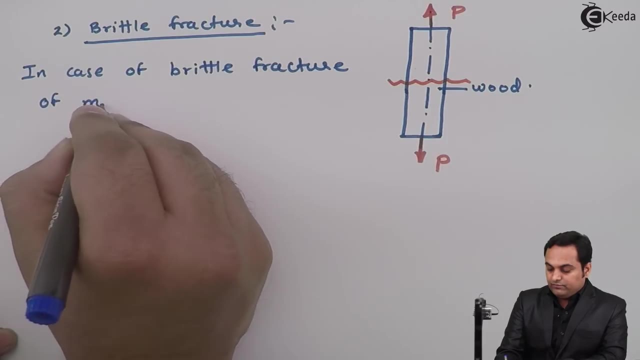 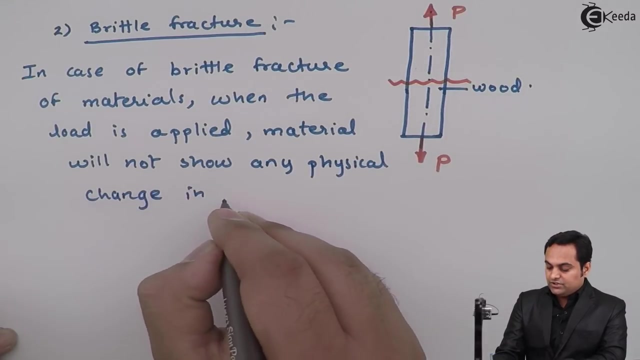 failure. so here I can say that in case of brittle fracture of materials, when the load is applied, material will not show any physical change in shape at first. so when the load is applied the material won't show any change of shape at first, or we can say initially: but 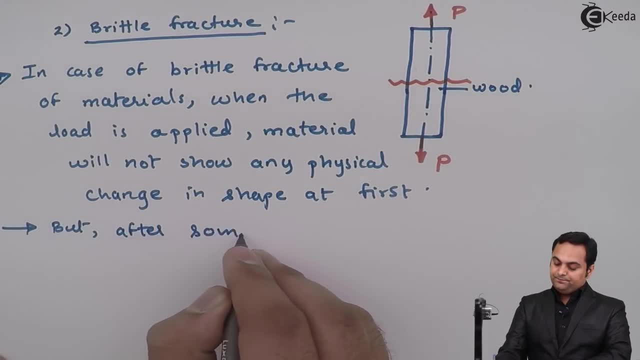 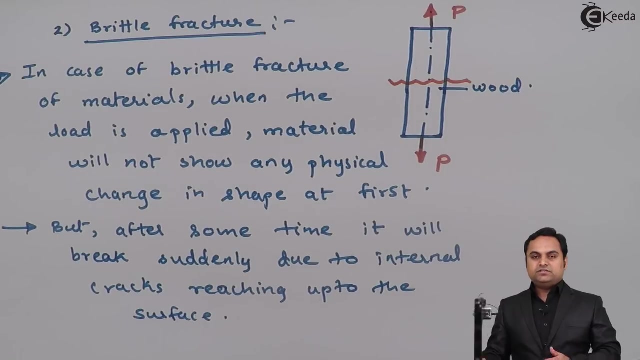 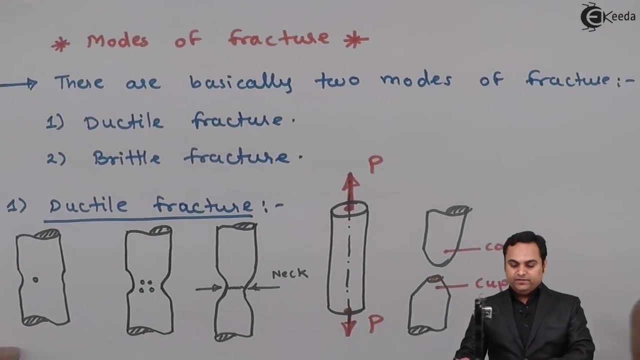 after some time it will break suddenly due to internal cracks reaching up to the surface. so in case of brittle materials they are not as easily. they will flow, as compared to the ductile materials previously which we have seen. in case of ductile materials we have the shape. 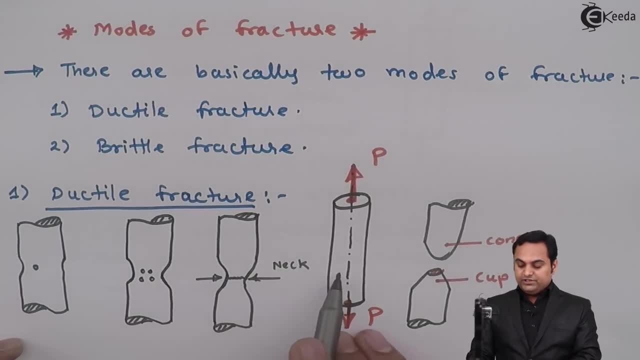 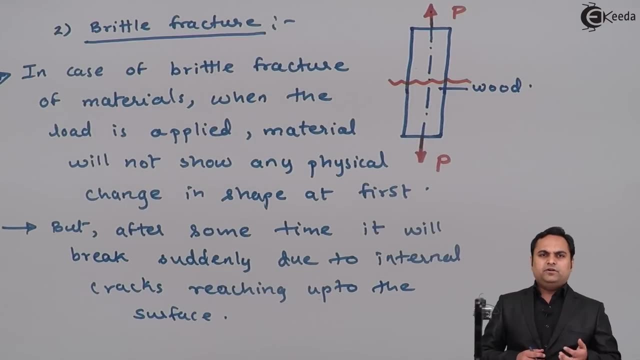 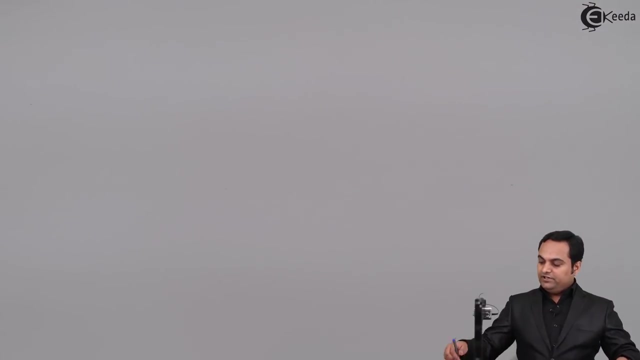 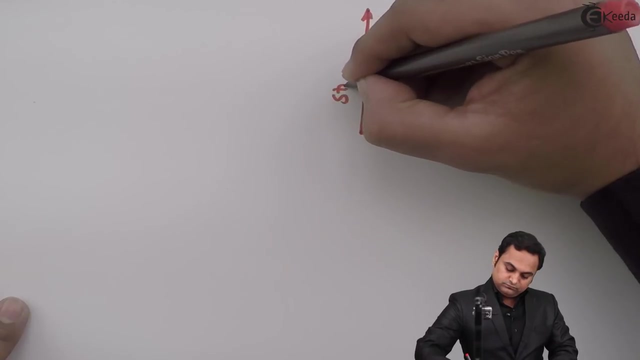 change was visible, that the diameter was going on reducing. it was visible and finally it failed. but in case of brittle materials, the material without any giving, giving any prior warning. it can break at any given instant. so I have drawn the graph for brittle material as well. 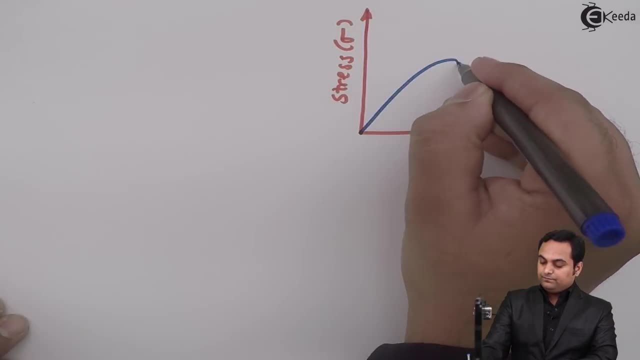 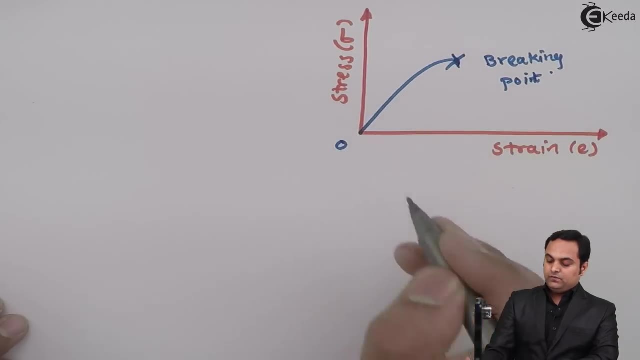 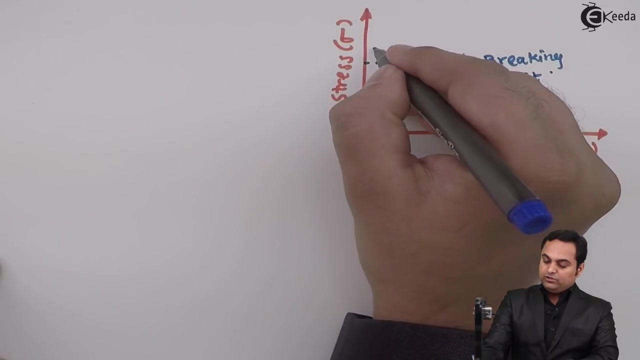 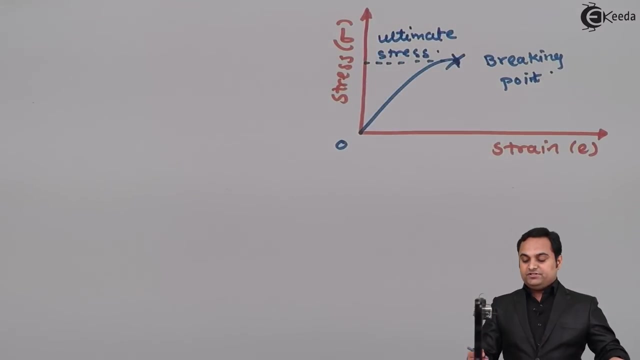 that is, the material will break directly without any giving any prior warning, and the value of stress it is called as ultimate stress, that is, the stress at which the material breaks so brittle.